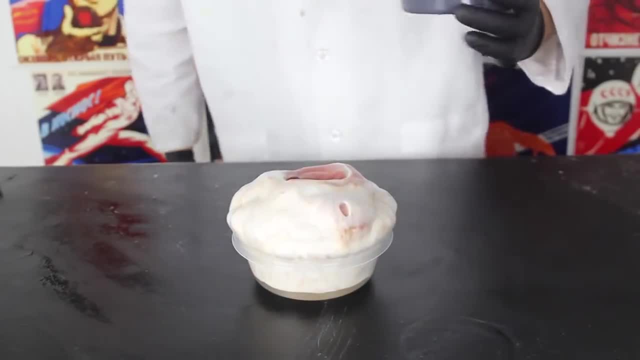 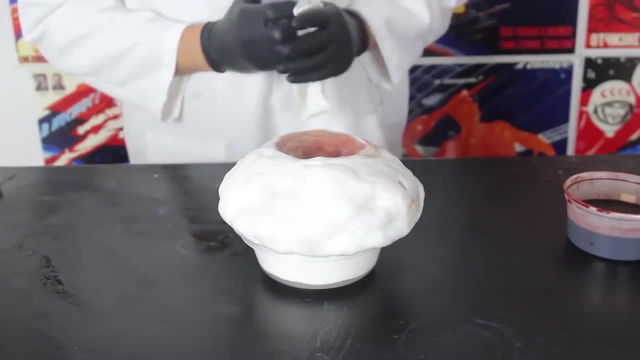 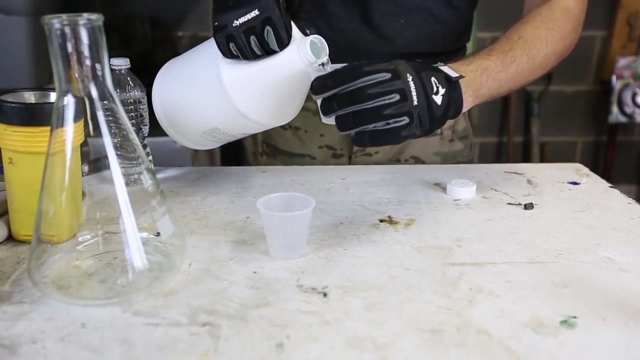 Pretty insane, huh. Same same thing. Just foam up like crazy. Looks like not much difference. Pretty much. 3% and 35% blow up pretty quick. First we're gonna get hydrogen peroxide- 35%- and fill it up with a glass, just like this. 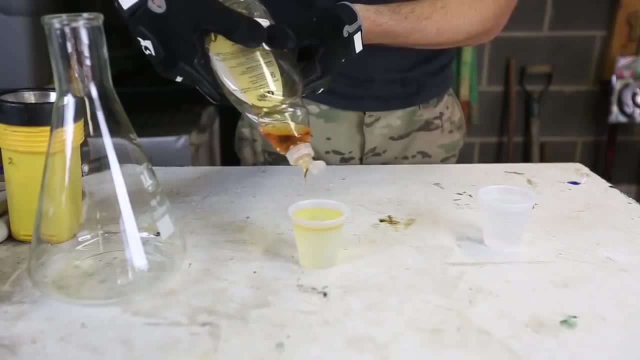 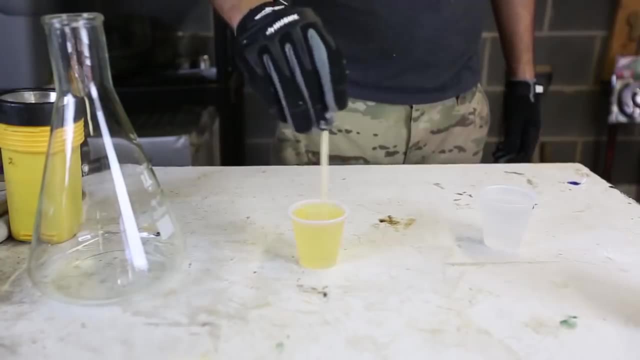 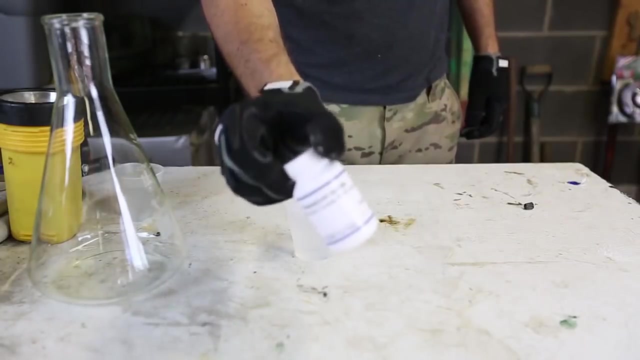 Boom, And then we're gonna set this aside. Also, we're gonna pour some soap into the hydrogen peroxide and then we're gonna have to mix it all up. Then we're gonna fill up another cup with water And we're gonna be using potassium iodide. 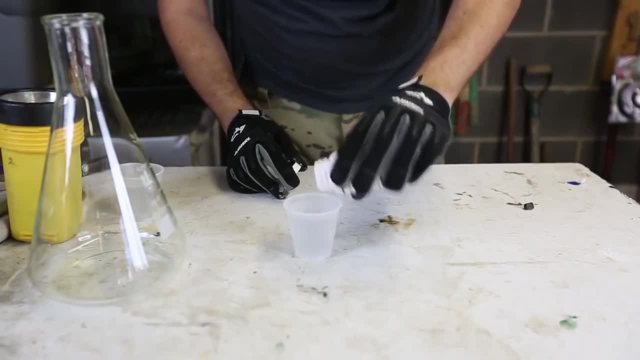 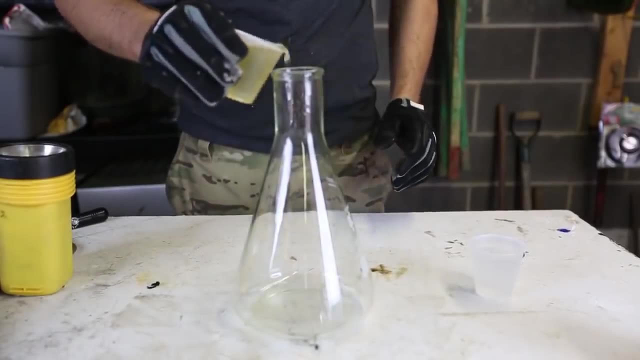 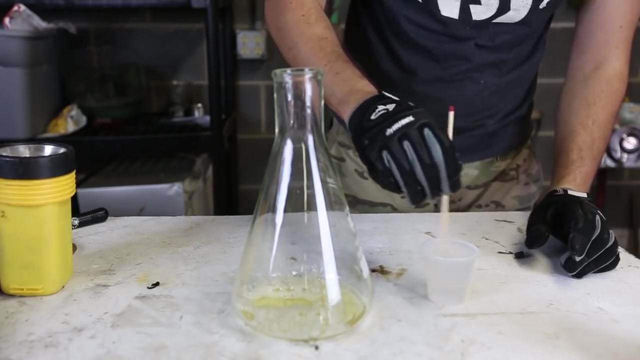 Pour a little bit of that- Crystals, Just like that. Then we're gonna grab one of these and pour this peroxide with soap. Boom, Just like that. Potassium iodide with water need to be mixed up really, really well as well. 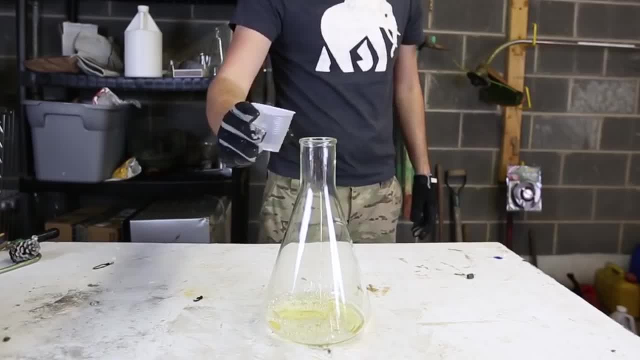 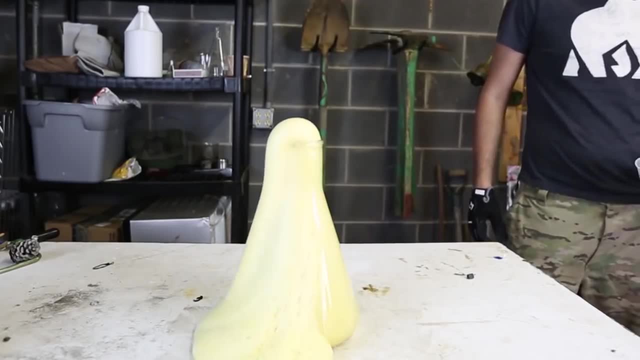 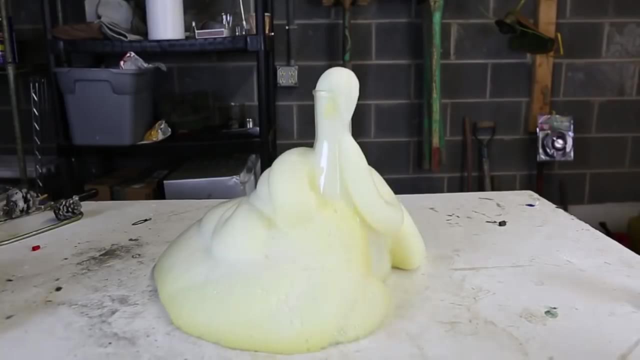 Now we're going to get potassium iodide solution and mix it together And let's see what happens. That's a lot of foam. What do you guys think? We're gonna try this again in a little smaller beaker, Got potassium iodide solution and hydrogen peroxide solution. 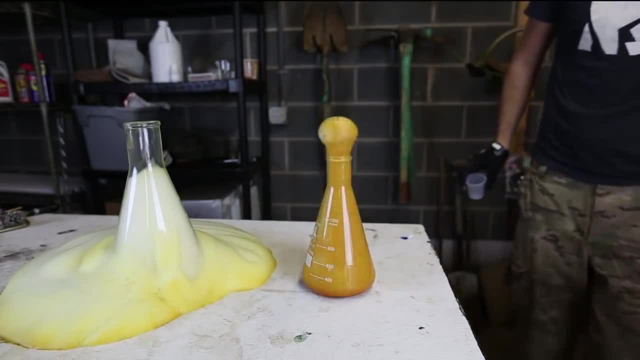 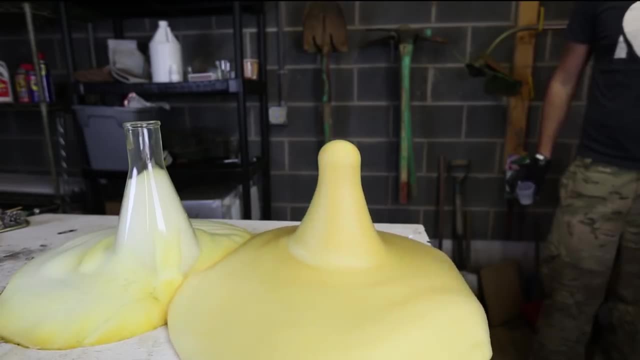 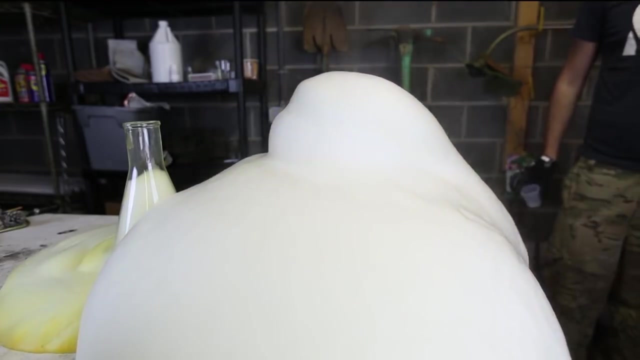 Pour it together. Look, it turns black. Whoa, This is insane. Look at this giant volcano foam: Whoa, This is Holy crap. No way, No way. What did I just do? That was way cooler than this one. 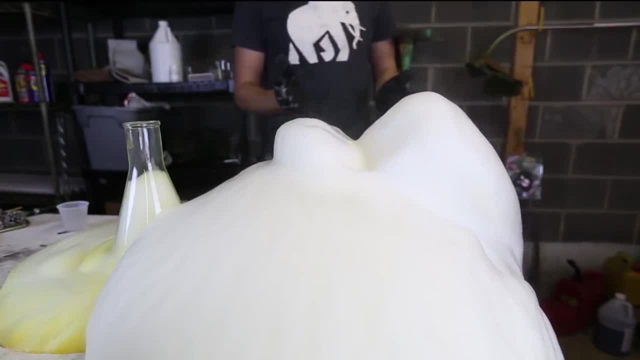 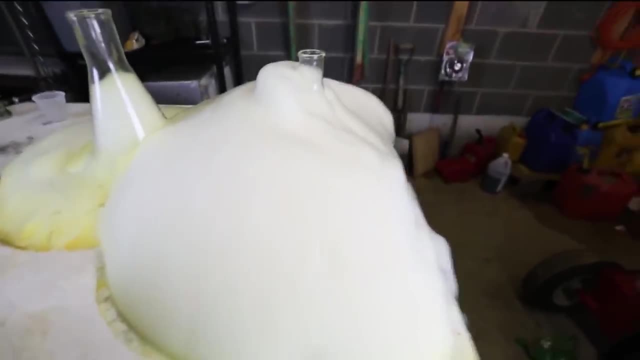 What do you guys think? I just needed a little bit more potassium iodide. This is insane Boom. Look how much foam Thumbs up for this experiment for sure. So this is what I'm gonna use. This is actually a Russian medicine. 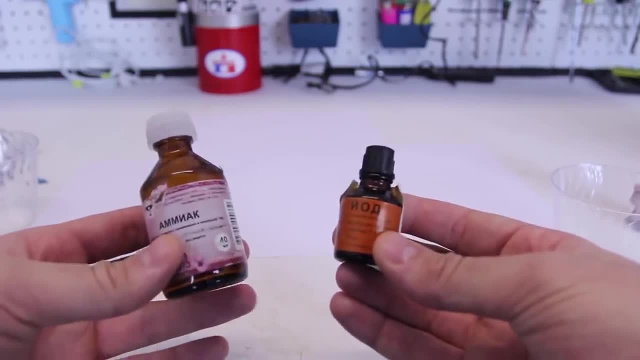 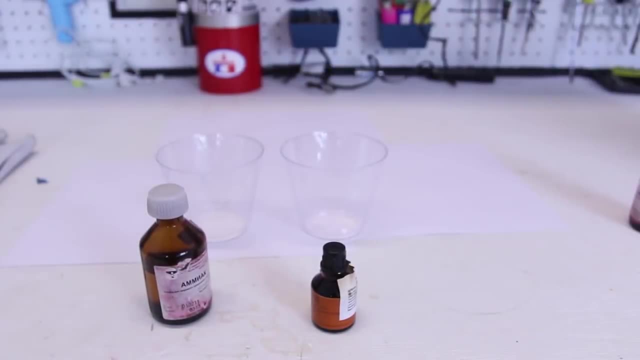 But if you mix together and dry it out, it's actually explosive. Let's check this out. I need two empty containers like that And a coffee filter. I got here two empty glasses right here. For this one, I'm gonna put iodine. 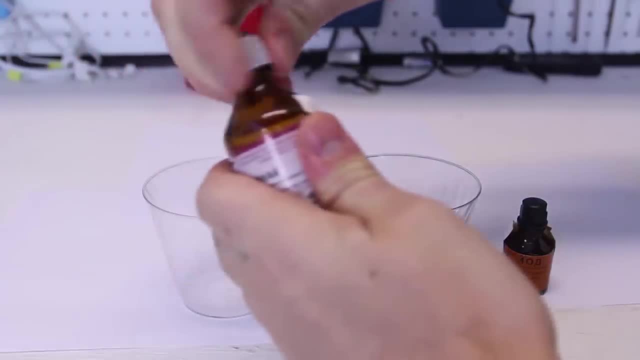 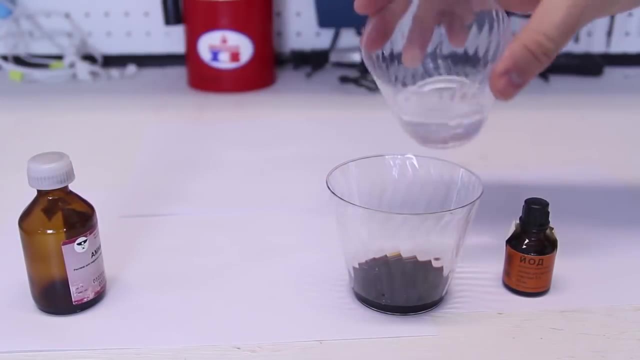 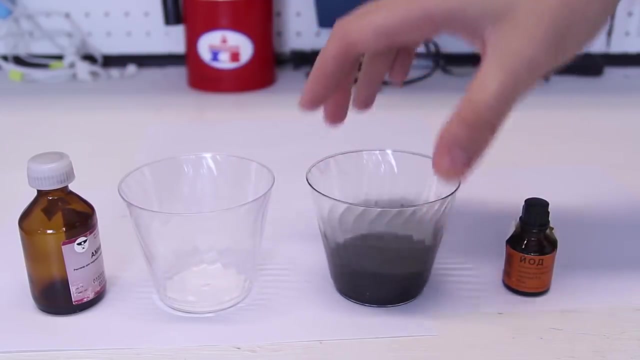 The whole thing. I'm gonna pour it in there. And here is IMEAC, IMEAC. in here The whole thing. Now I'm gonna, Now I'm gonna pour this one together And mix them up. You see how it turned- kinda black. 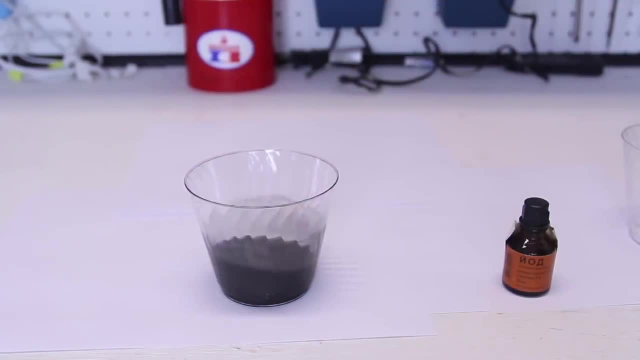 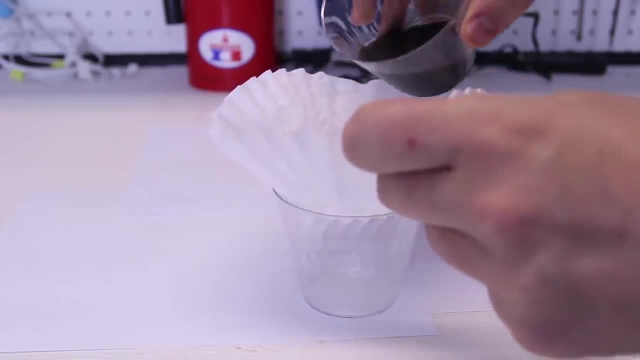 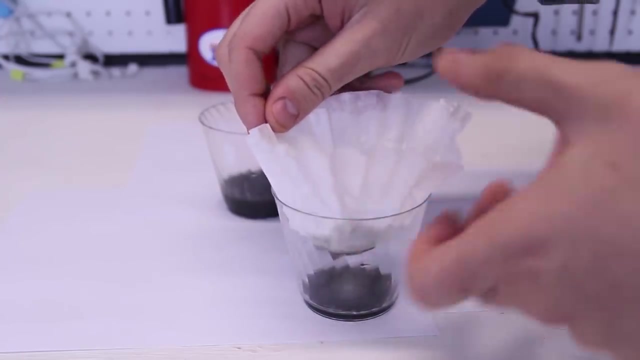 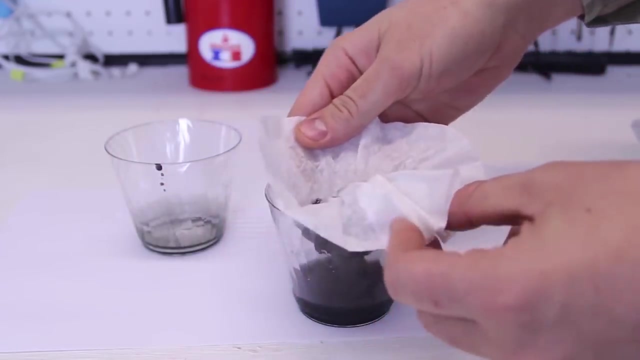 Now we're gonna let it sit for like an hour. Mmm, that thing stinks. Then I'm gonna need a coffee filter. Put it like this And just pour it in there. Just gotta wait till it all goes through. Okay, now I have to just wait till it just filter itself out in there. 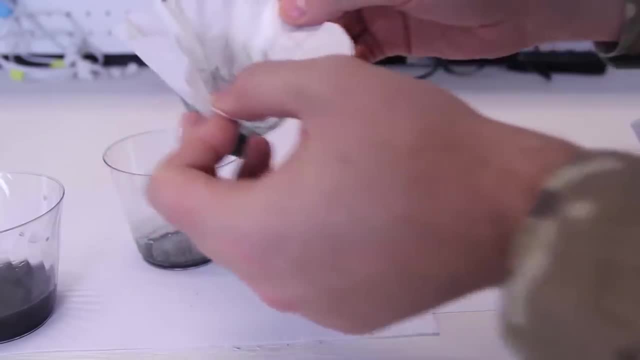 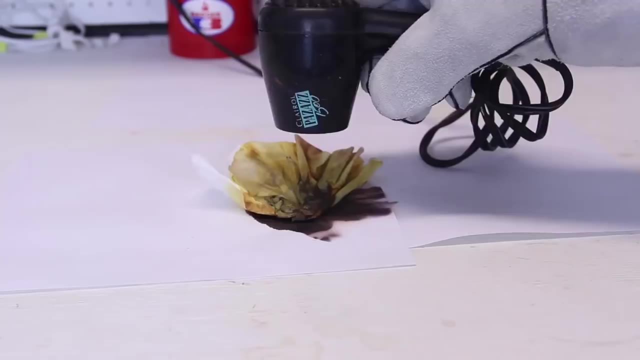 You see, it's like slow, Slowly going through. Now we're just gonna dry off that paper, Just gonna lay it down here And let's see what happens. When it's finally dry, we're gonna grab a hammer and see what happens. 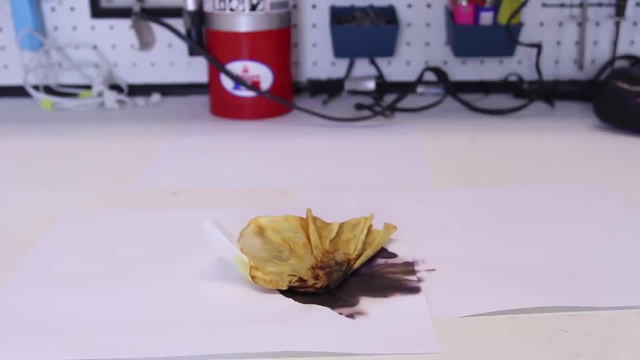 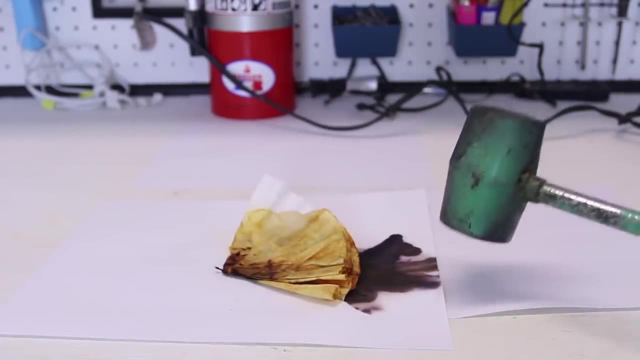 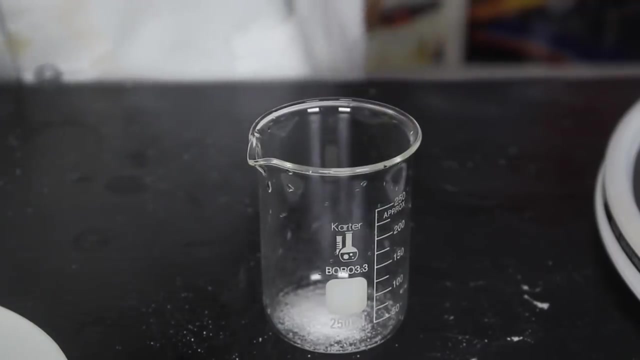 Crazy huh. And this is very, very light touch. Let's see Pretty crazy huh, Exploding paper. First thing we're going to do is Put a little bit of borax in there. Very little bit, Just this much. 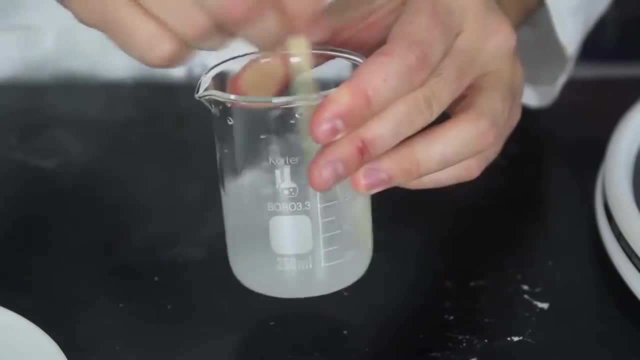 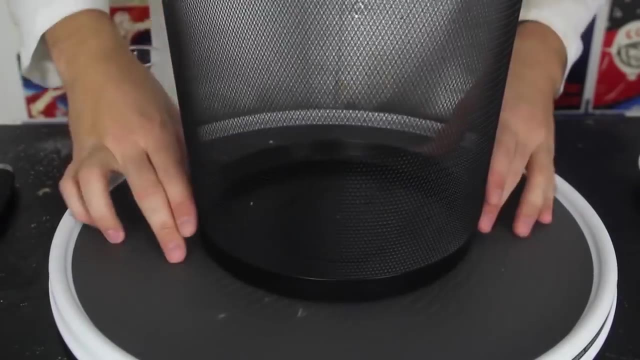 And then we're gonna pour ethanol, Now we're gonna need to mix it all up- Kids, do not try this at home- Then we're gonna bring this pinion tray back And this garbage bin And we need to find the center. 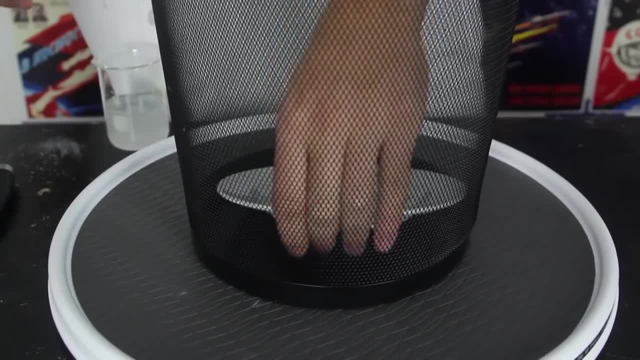 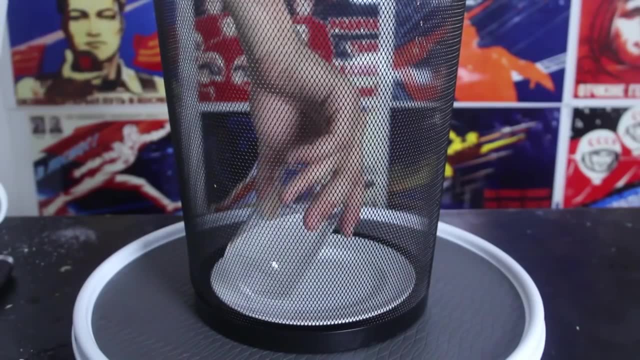 This is close enough, Then we're gonna put a plate in the middle. Now I'm gonna grab some of that mixture And put it in there- Not too much, Because I don't want to spill it So very little bit. Now I'm gonna shut down all the lights. 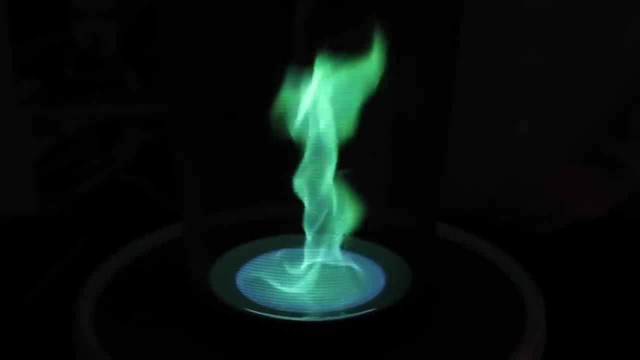 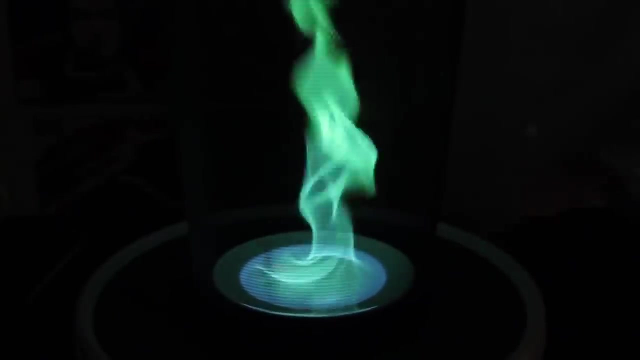 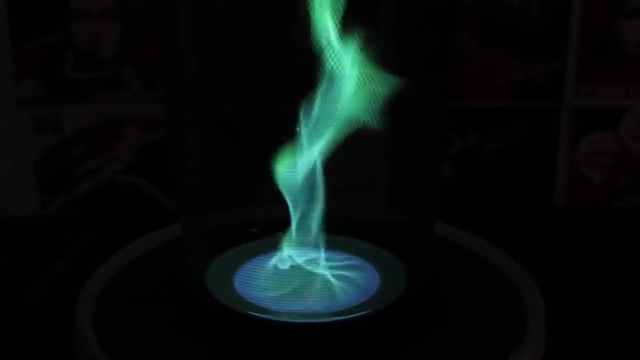 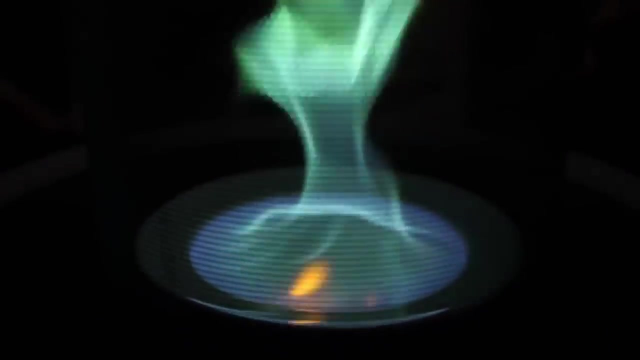 And now we're gonna spin it And we're gonna get fire, Green fire, tornado. Look how beautiful. it is Pretty amazing. What do you guys think? Let's do some close up Some of that, Focus it And let's see if I spin it. 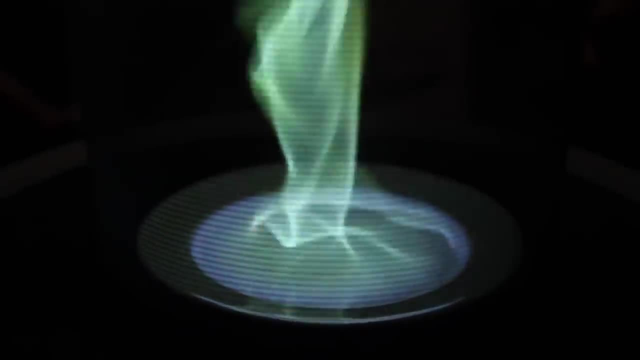 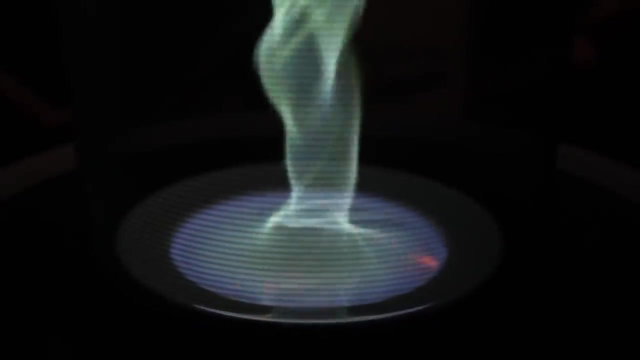 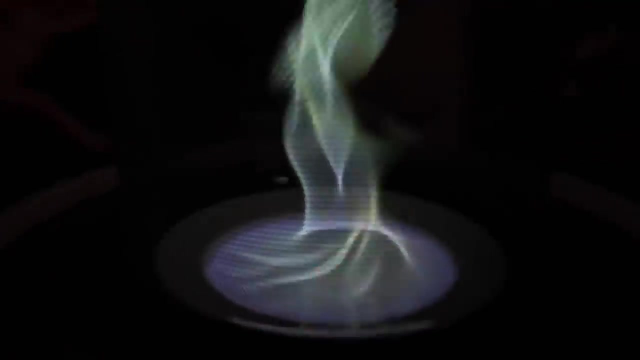 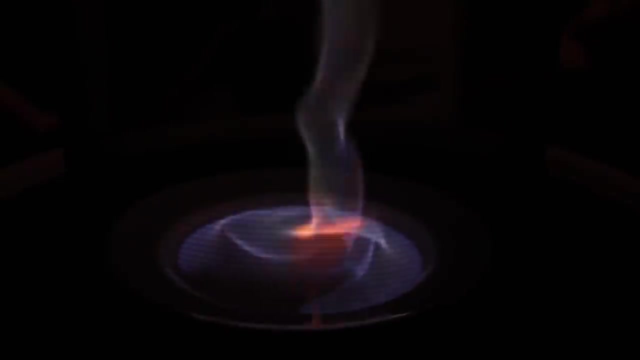 How amazing is that? If you want to see it in slow motion, subscribe to Slow Mo Lab, Maybe I'll do it next video. Pretty amazing, right? And you see borax wearing out And now it's becoming blue fire. So right here we're going to need instant light powder. 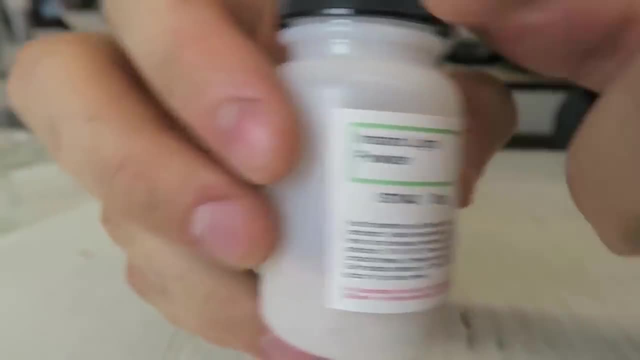 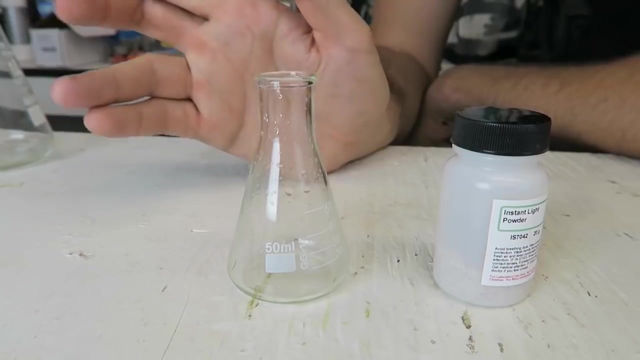 Look at this- Pretty awesome, So I got it online. We're gonna need one of those little tubes And we're gonna make a really cool experiment. Let's check this out First. we're gonna fill it up with water in a beaker. 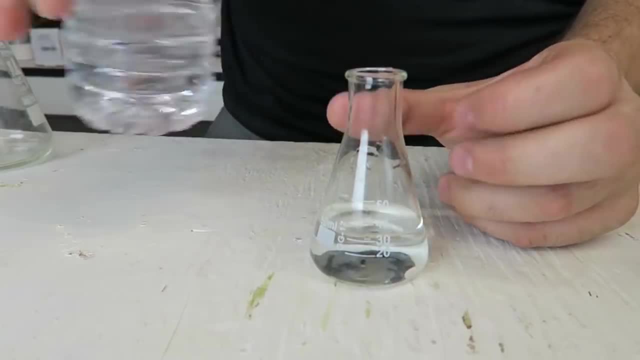 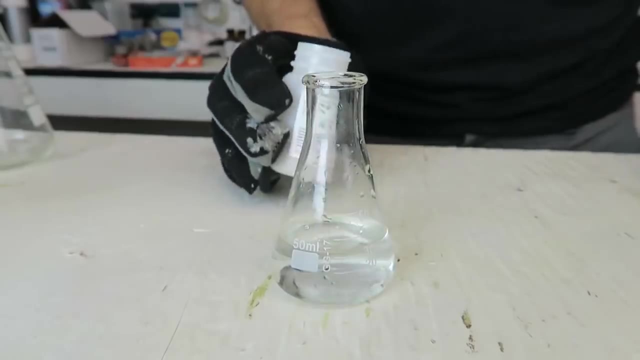 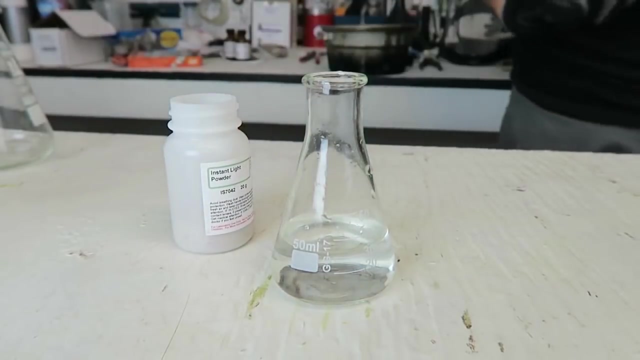 It's a distilled water or natural spring water. We're gonna fill up about 40 ml of distilled water Just like this. Then we're gonna grab our instant light powder And pour it in there, But first let's turn off the light so we can see the reaction. 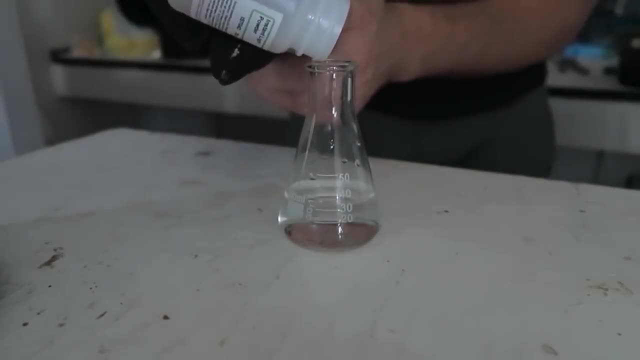 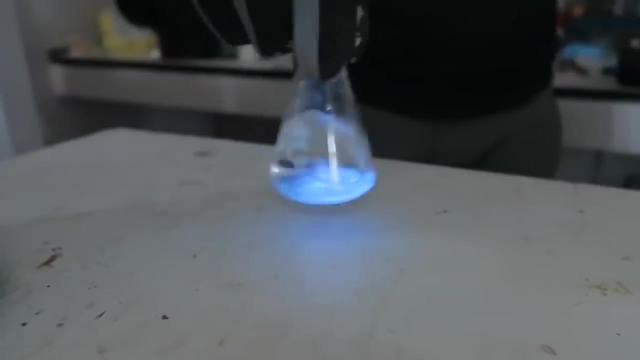 So we're gonna pour this stuff in there About a few grams, Like 3 to 4 grams, And look, it's already starting to light up And if I mix it- look at this, We're gonna mix it. Look how crazy it is. 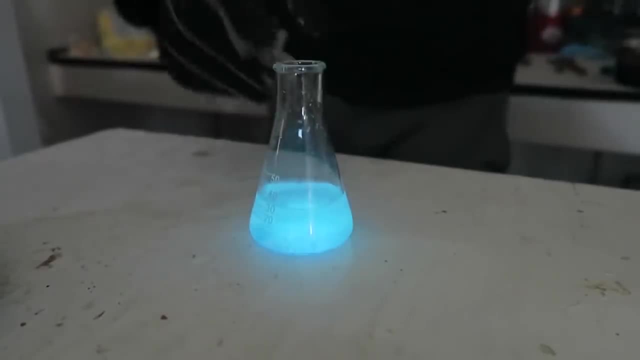 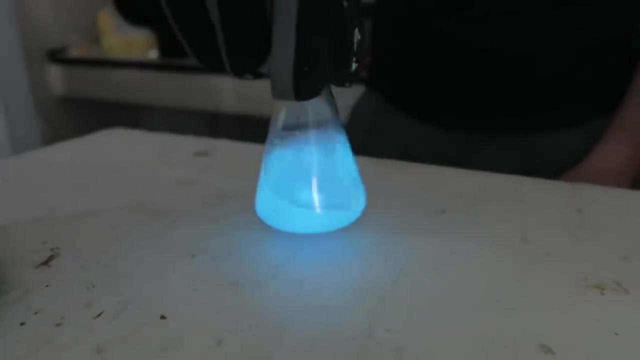 Look how lights up it is. Wow, That's insane. I bet they use that in movies. Look how beautiful it is. Isn't it insane how beautiful it is. It looks like it's not even real. It looks like a glow stick, but it's not. 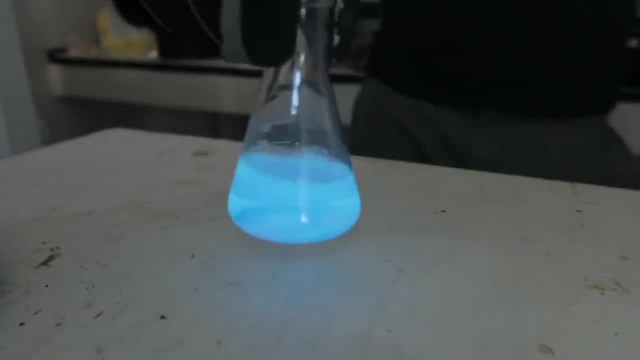 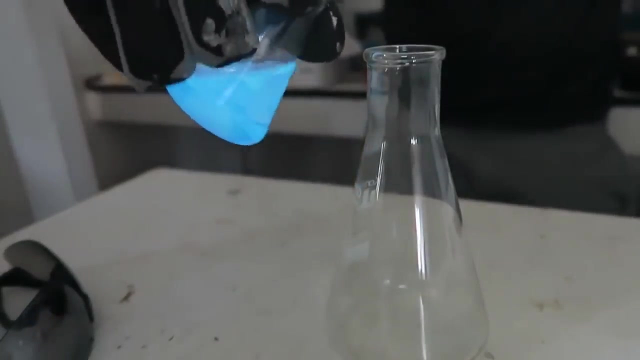 Look at this beautifulness, Amazing, huh. We should pour it from a beaker to another beaker. I bet that's gonna look cool too. So I'm gonna grab this part, This glow in the dark, This liquid, And pour it in here. 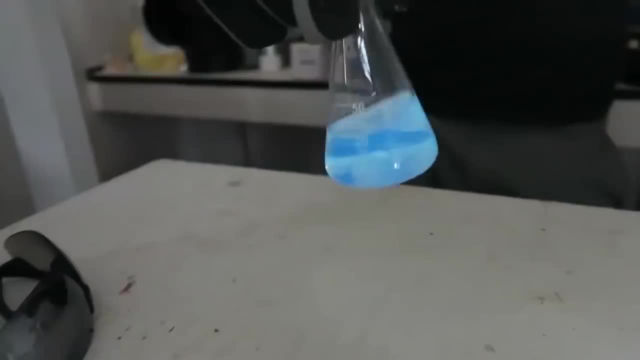 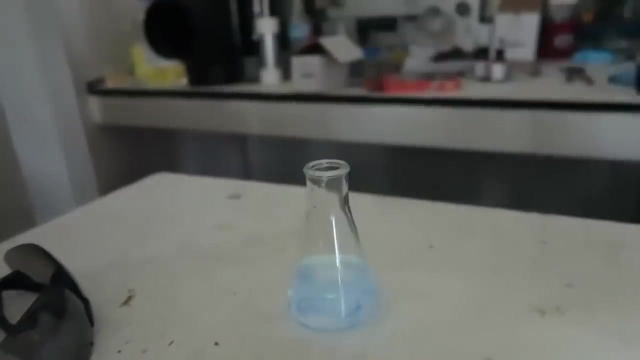 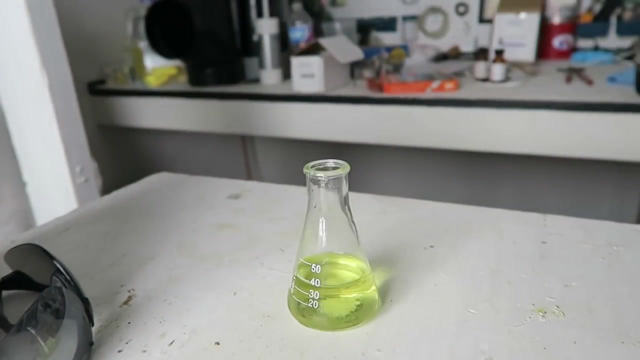 Whoa, Look how awesome it is. Now let's see what it looks like, not in a dark room, but very light up room. Let's check this out. Wow, You see, as soon as I turn the lights on, instead of blue color it looks like yellow color. 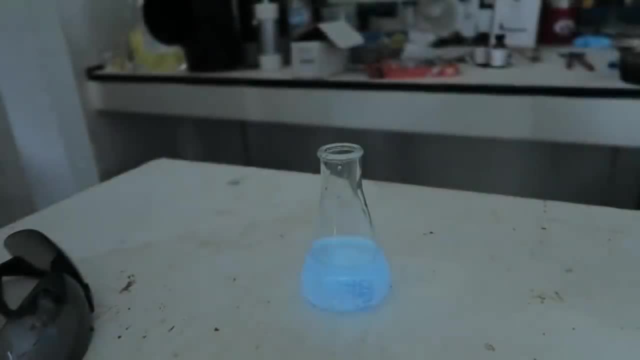 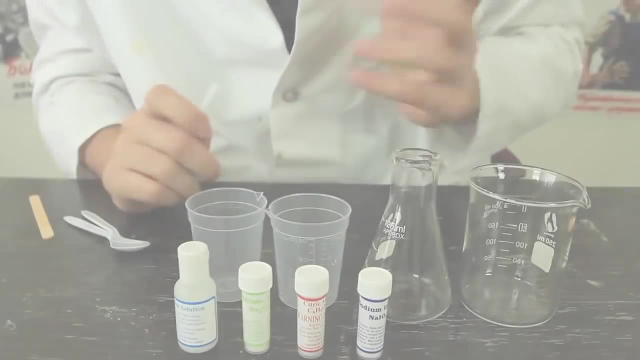 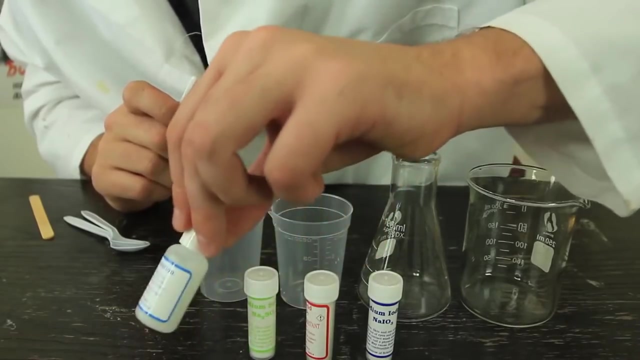 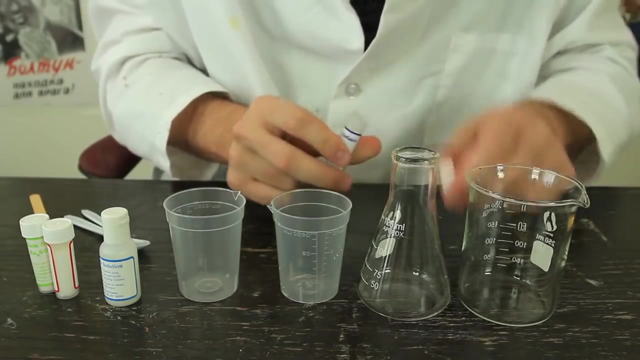 Pretty amazing, huh? Look, It's light up again. How beautiful is that? So we got here four chemicals- Sodium iodide, citric acid, sodium sulfide and starch solution- And we have here two mixing containers And what I'm gonna do is grab sodium iodide. 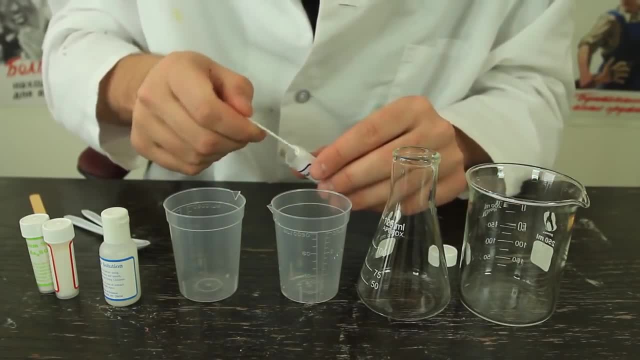 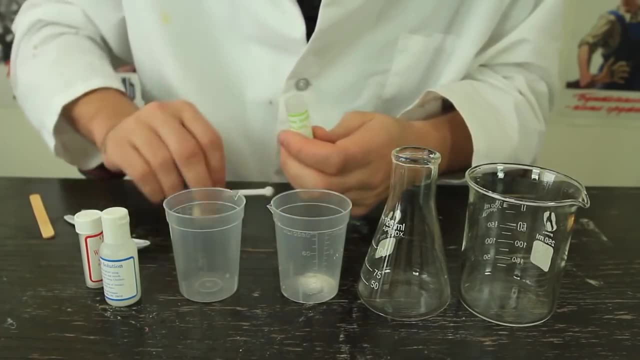 And grab one small spoon, Like mini spoon, Like that, And drop it in there. Then I'm gonna grab sodium sulfide- Half a spoon or half of small spoon And put it in there. Then we're gonna grab citric acid. 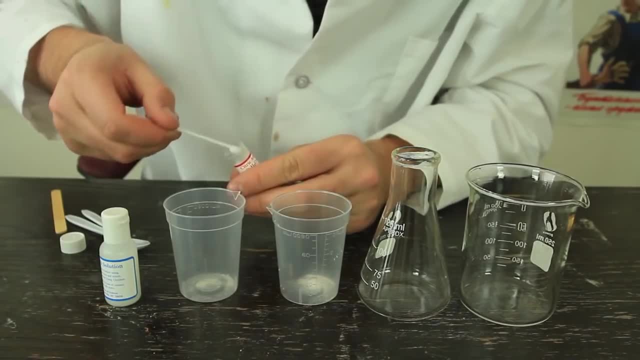 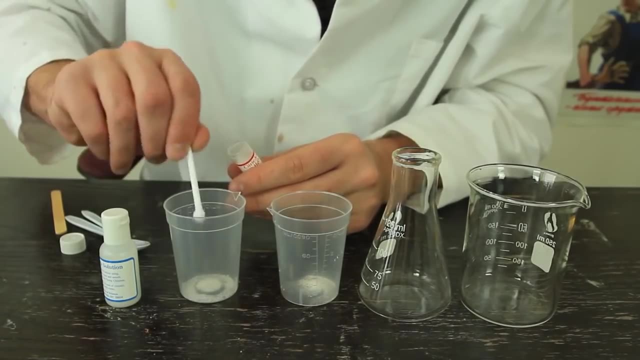 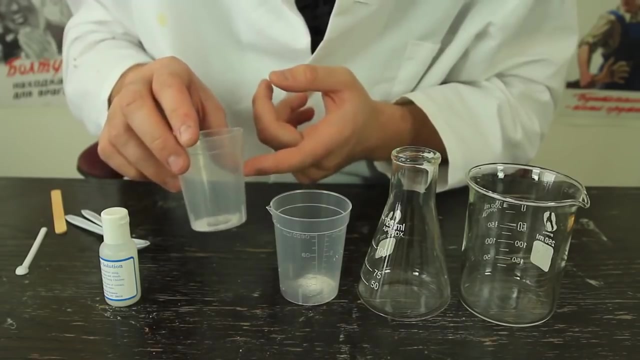 And grab two small full spoons of citric acid, One And two, Then we're gonna need warm water to mix it all up. Each about 20 milliliters, But if you wanna do like twice the amount, like twice bigger. 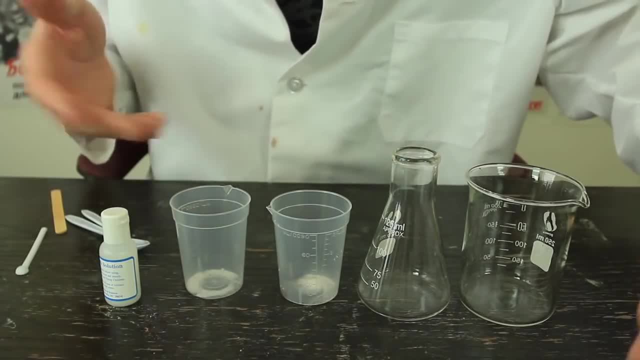 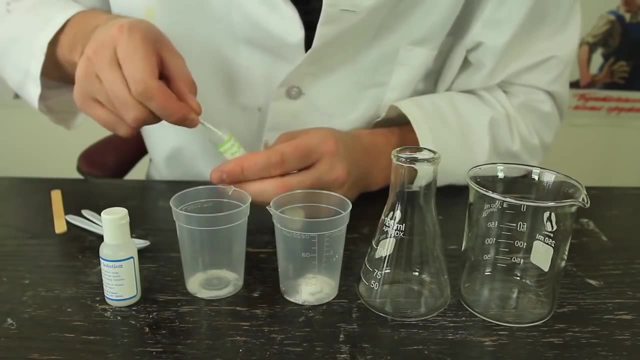 or, if you wanna do, 40 milliliters. so we have to put same amount in each. Like what was it? It's sodium iodide, one spoon, Half a spoon sodium sulfide And two more spoons of citric acid. 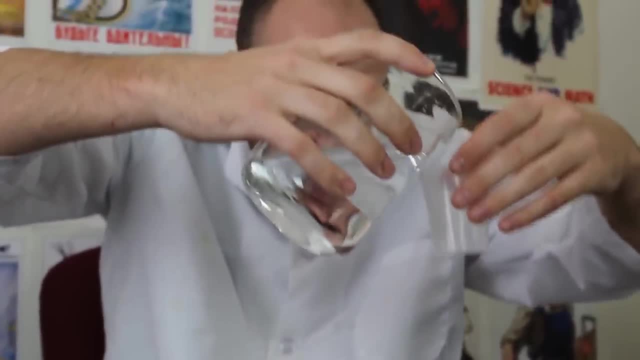 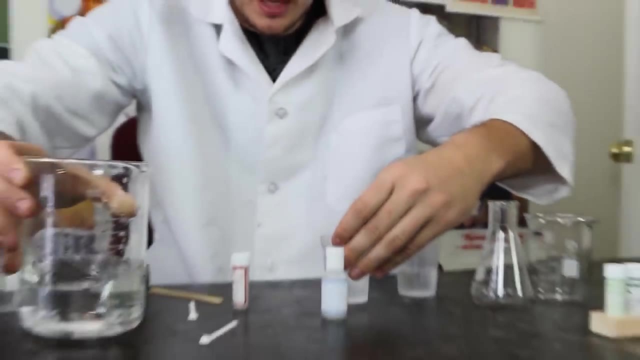 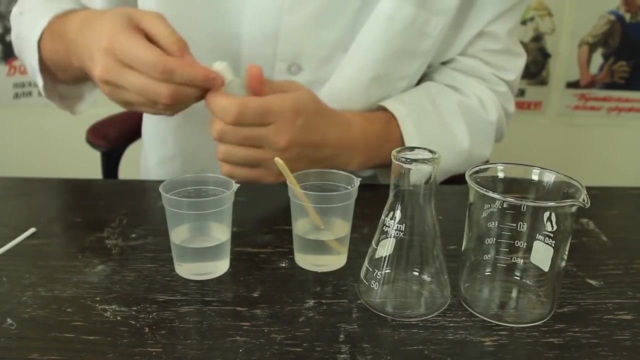 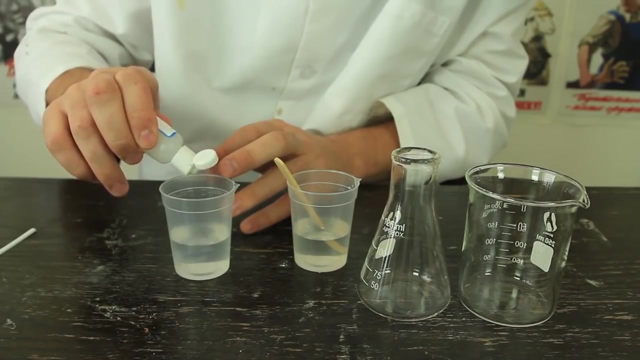 Here And here. And 40 milliliters of water here, Just like that. And When we put the sodium and citric acid, we're gonna put: uh what, six to eight drops: One, two, three, four, five, six, seven, eight. 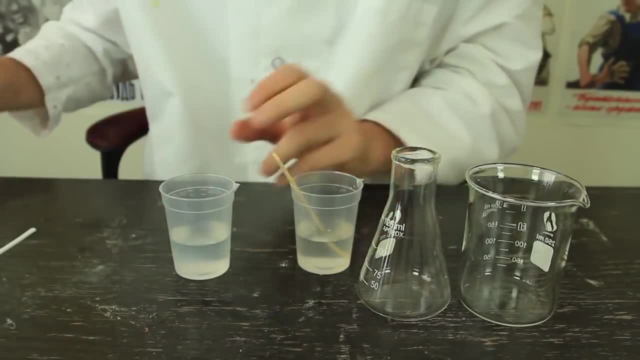 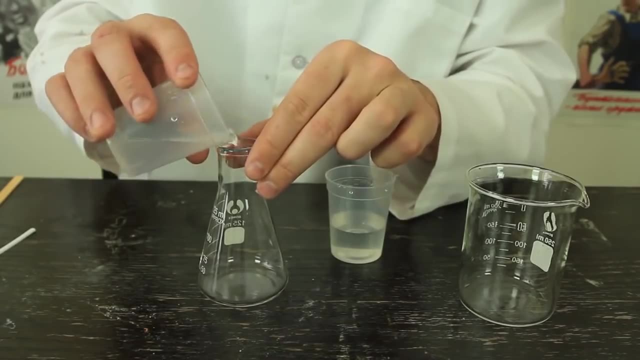 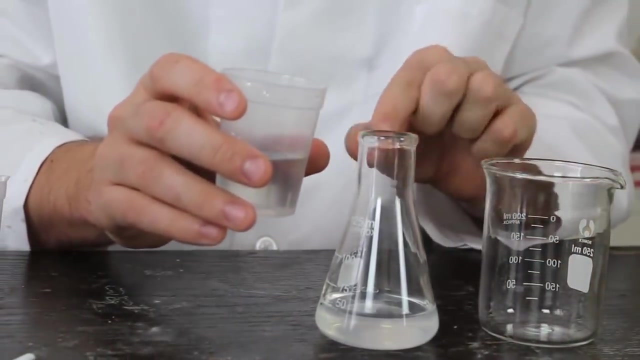 Then we're gonna need to mix both of them up. Okay, after it looks like it's mixed, we're gonna pour one solution in here, Then the second one, And once I'm gonna pour it in there, I'm gonna start pouring it in here. 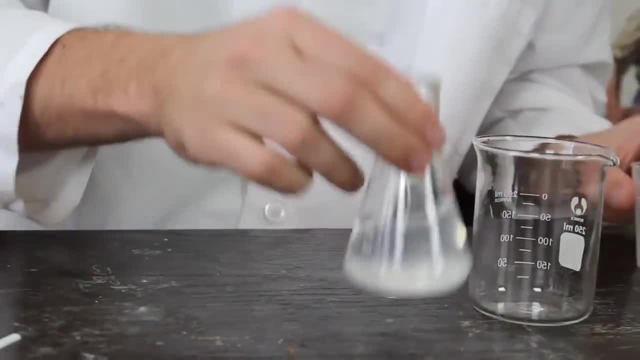 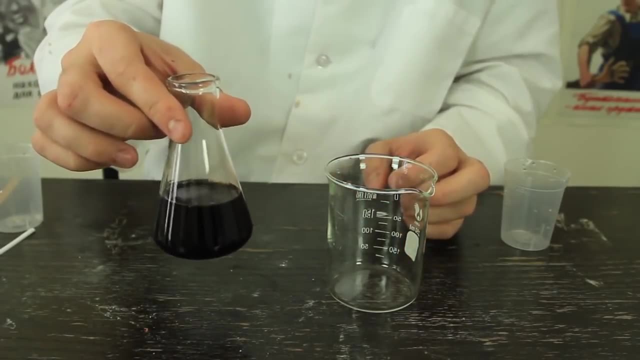 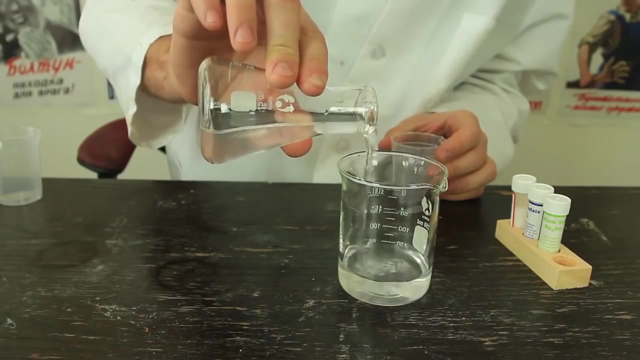 Let's see what happens. I'm gonna mix it couple times. Ooh, Did you see that? I'm gonna mix it couple times. Ooh, Did you see that? Whoa, Ooh, how cool was that? Amazing, huh. 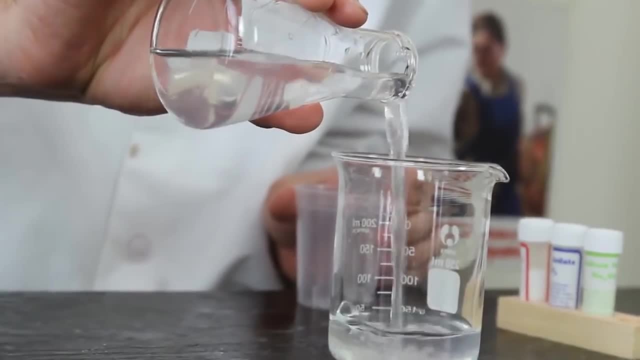 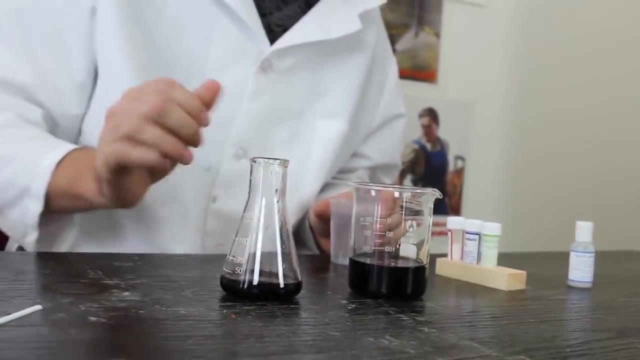 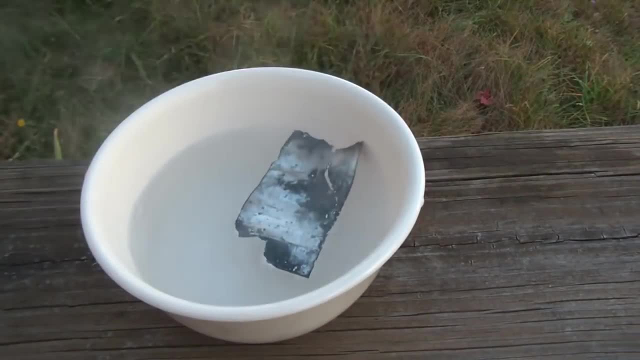 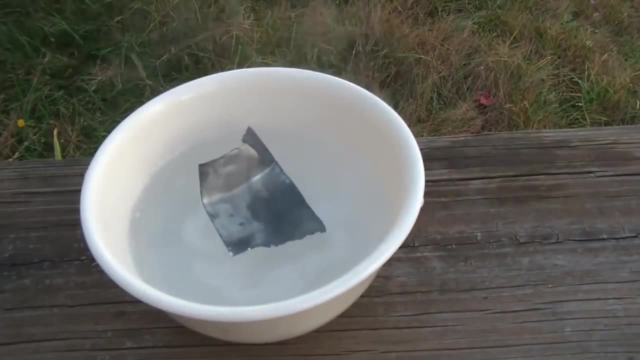 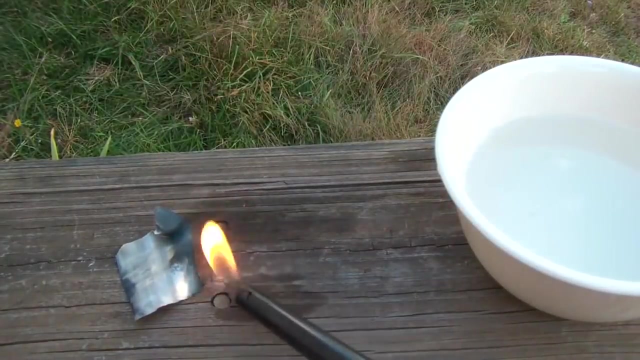 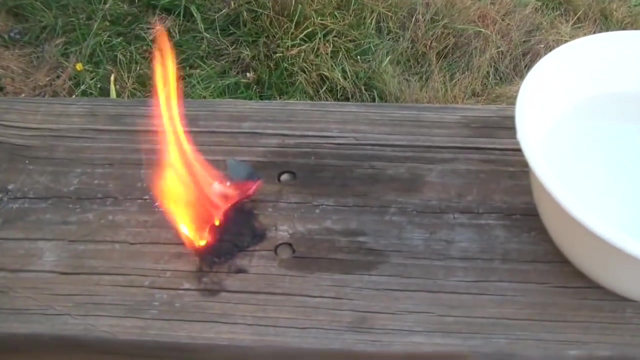 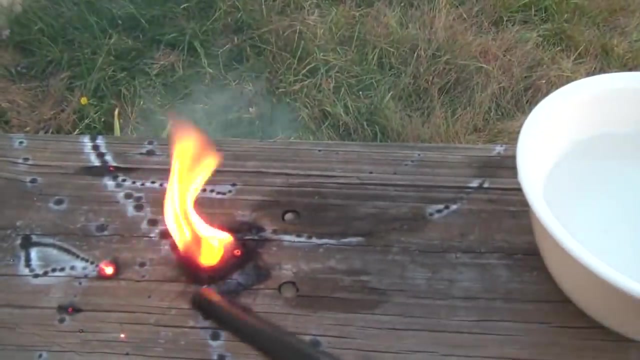 and throw it in water. See what happens. See what happens. Actually boils, Actually boils. Now we're gonna turn something different. Try to burn it small piece. First we're gonna put powdered sugar, then we're going to pour sulfuric acid in there. 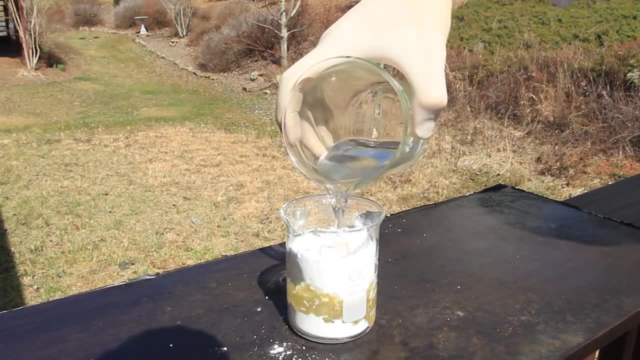 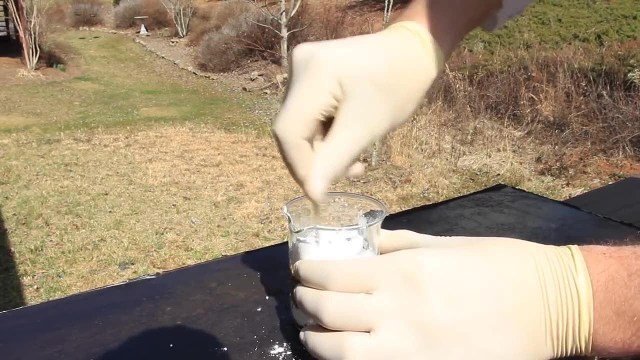 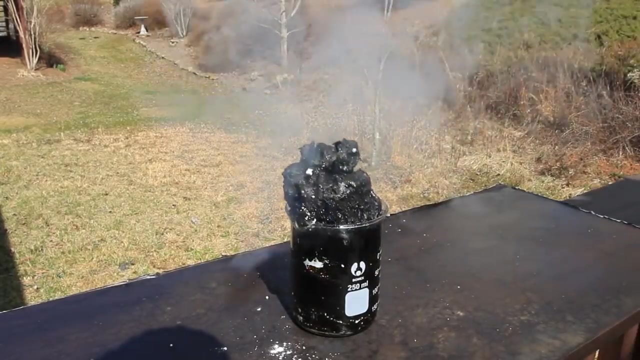 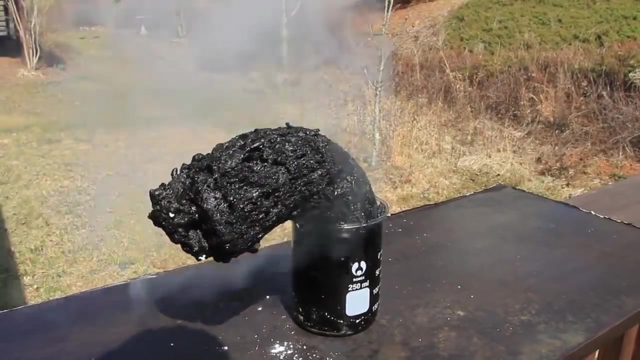 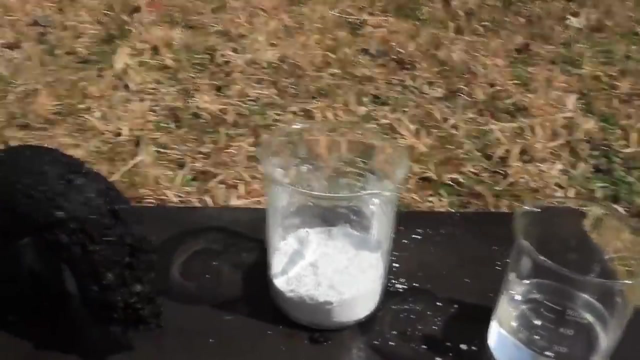 Then we're going to pour sulfuric acid in there. you see the reaction already starting. so what you're gonna, what we're gonna do, is mix it up. I think it got so hot that the glass even popped- but how crazy is that? so we're going to dry this. 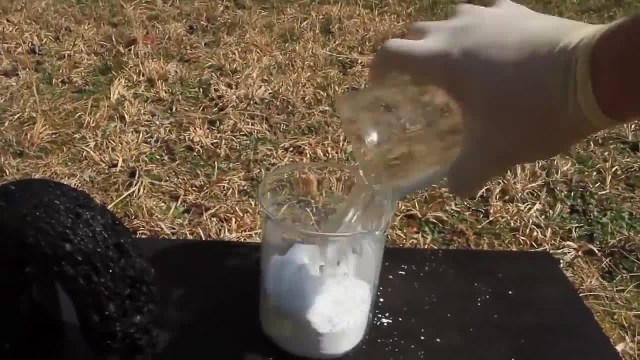 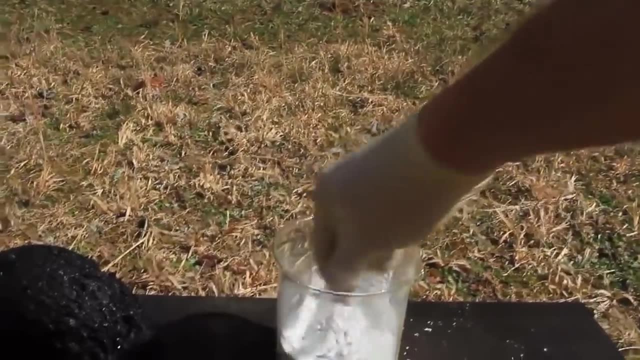 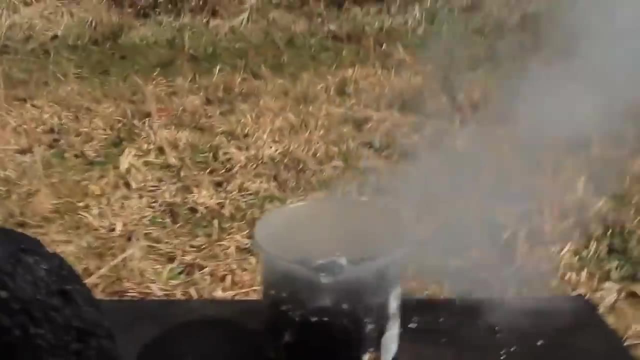 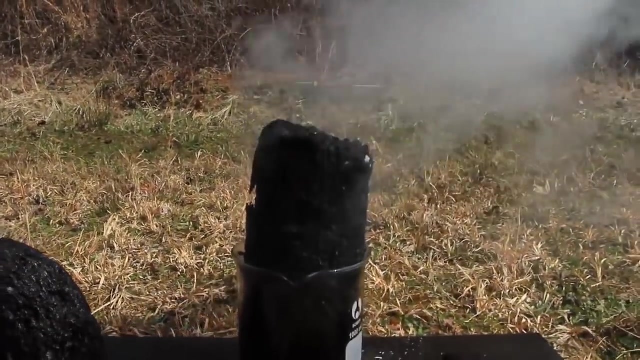 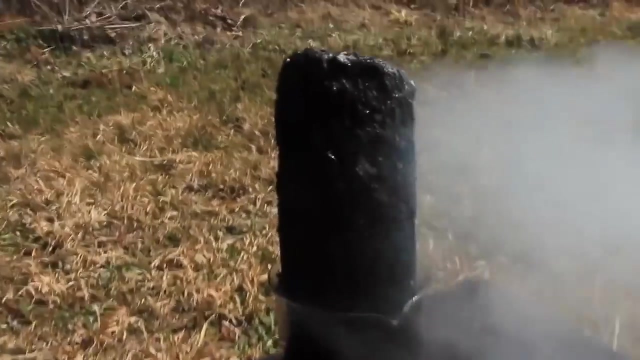 again, but on a bigger level. so we're gonna put sulfic acid in there, and then we have to mix up this sugar shoot. that's a thick one right here. how crazy is that? just keep coming and coming. experiment with the sodium acetate and water. well, what do we get? 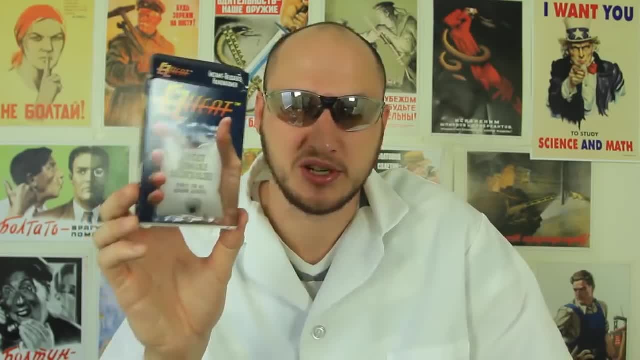 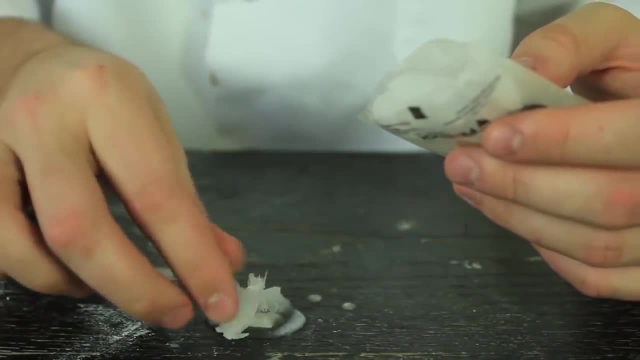 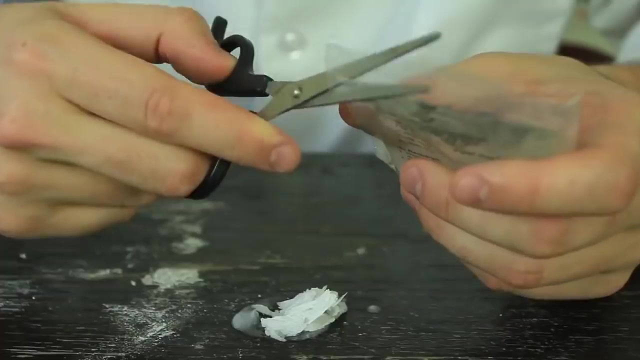 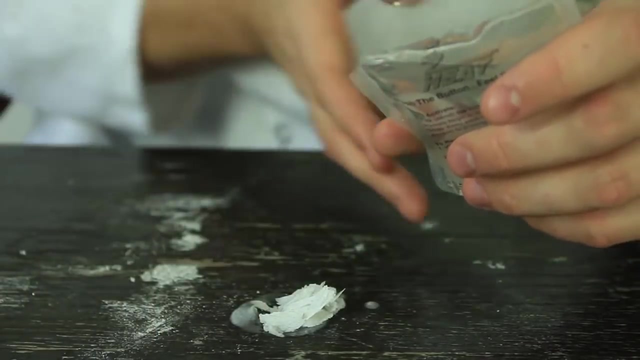 sodium acetate, easy heat hand warmer. so here's the use one. what I did it is open it and grab a piece out of it. I'm gonna put them in here, you know, just like that. so then I'm gonna cut it right here. look you see how careful I cut it and now I'm gonna put on this crystal and 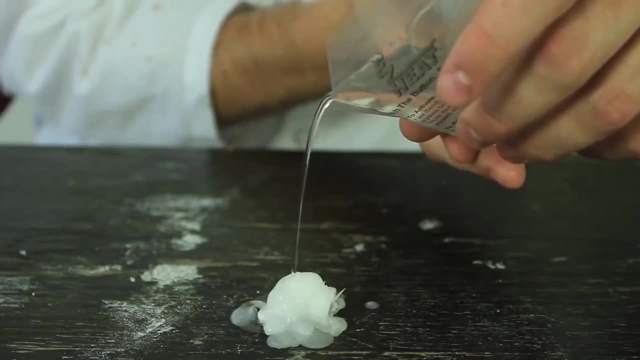 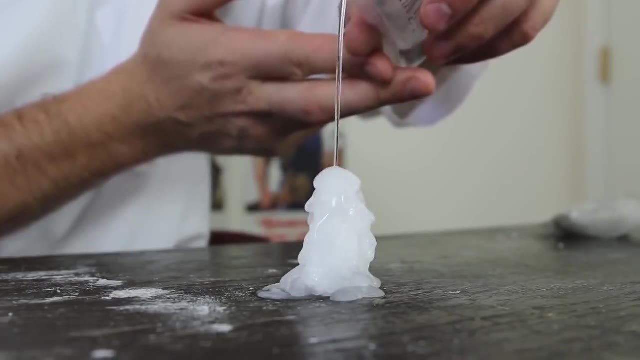 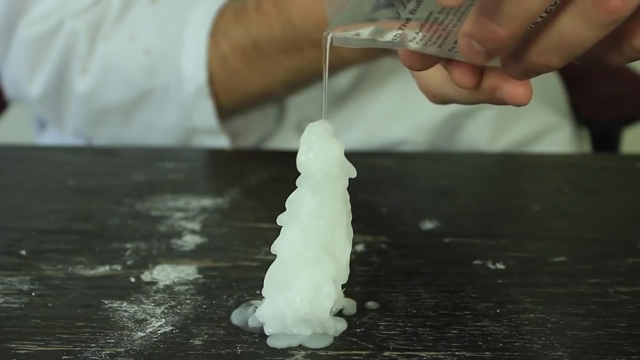 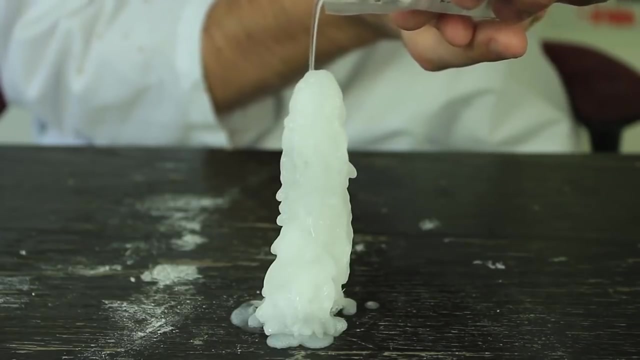 let's see what happens. how cool is this? okay, I guess I'll show you how cool this is. okay, I guess I'll show you how cool this is. you just crush the ice right away, and this thing is super hot and warm. so I got you a couple of chemi's right here. I'm gonna put that one right here. 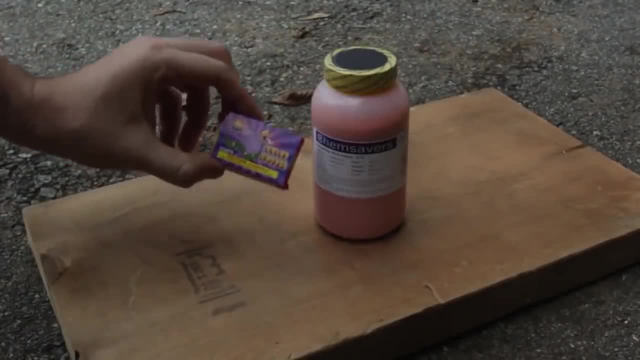 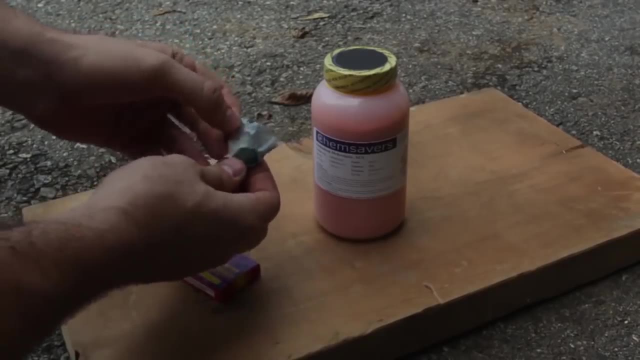 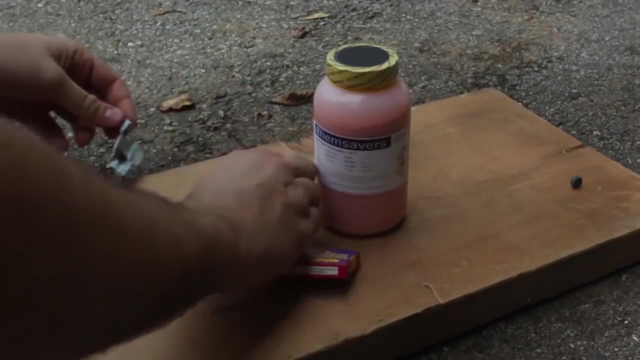 Ammonium Dichloride. And then I got here Black Snake. See in the description What kind of chemicals this firework contains. So this little black type tablet, Just like this, I'm gonna open them up And lay them like this on a board. Then I'm gonna grab Ammonium Dichloride. 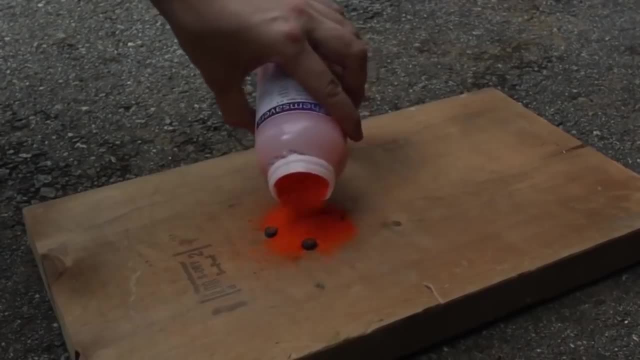 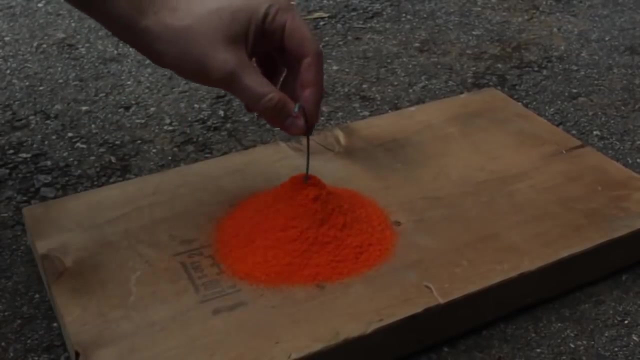 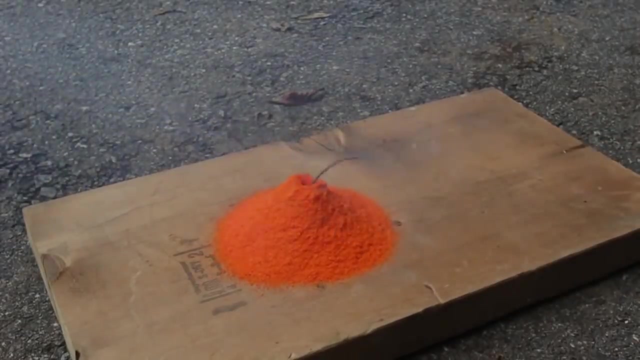 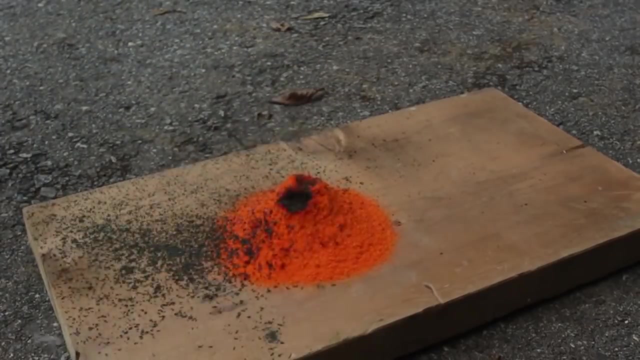 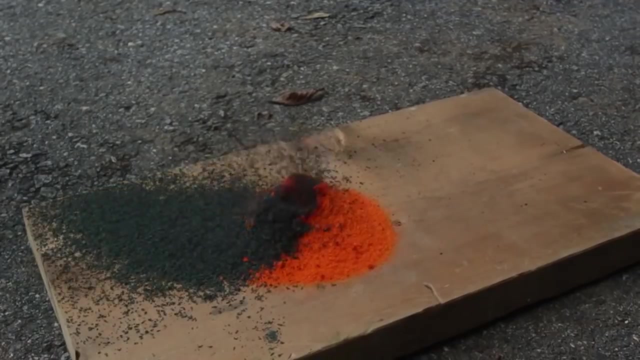 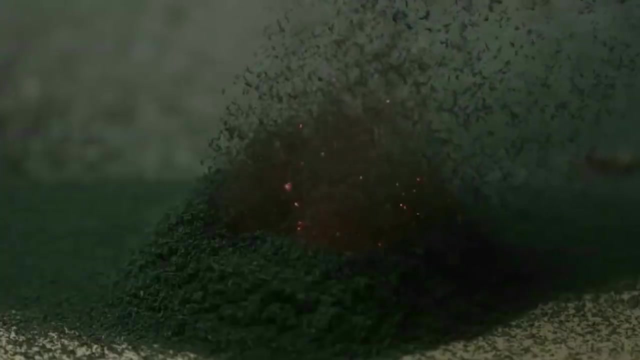 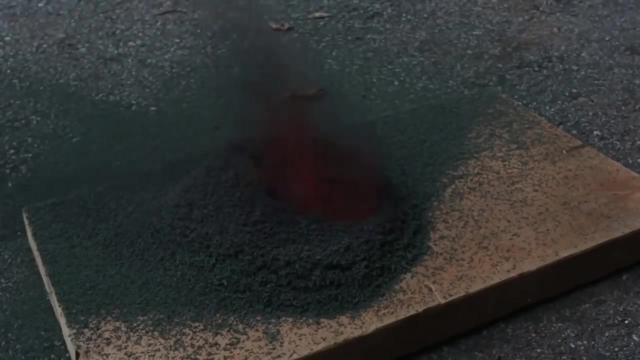 And just put it right on top of them, Just like this, Something like that. Then I'm gonna grab a fuse And stick it Right in the middle of it. Okay, let's light up the fuse And see this beautiful reaction. Pretty amazing, huh? Look at this. Looks like a volcano. 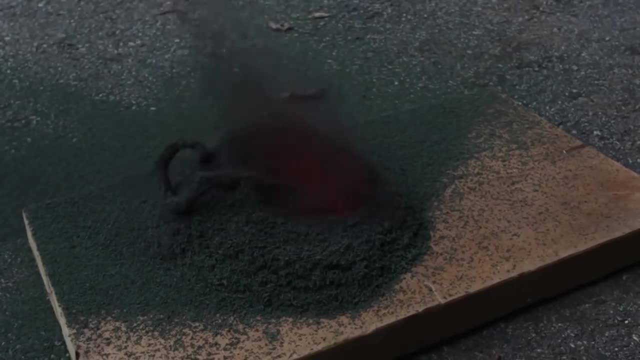 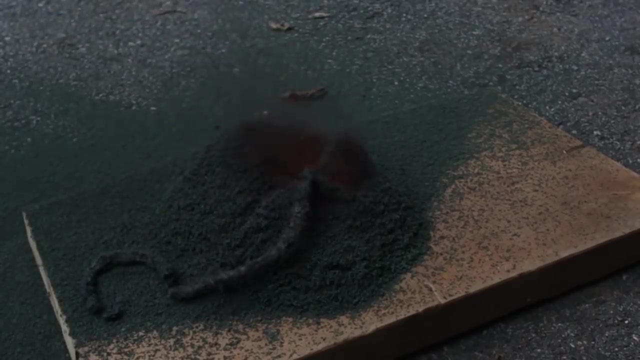 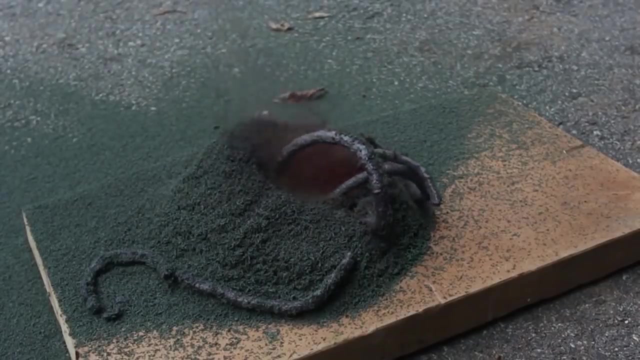 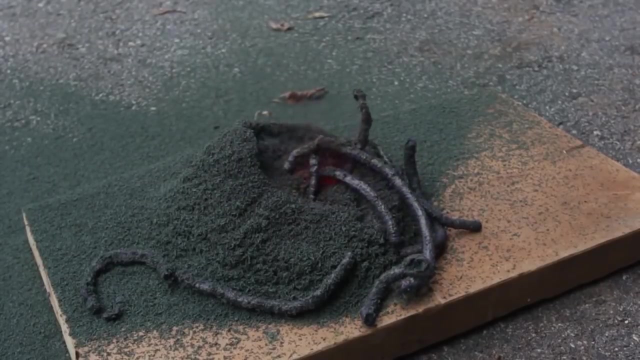 But let's just watch When the snakes comes out. Check this out. Look at this. Look how creepy this Looks like a demon coming out Out of the earth. Look at this- black worms Coming out- Pretty insane. I gotta try this again. This is beautiful. Wow. Look how much ash coming out. 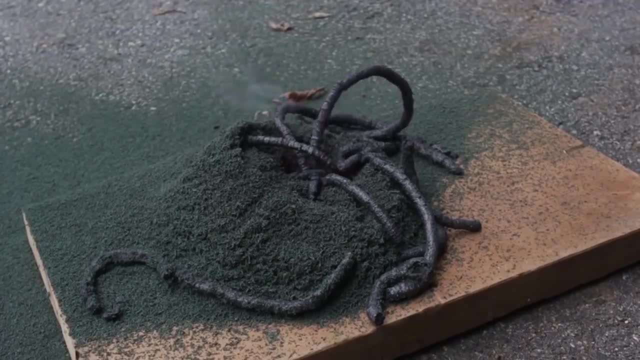 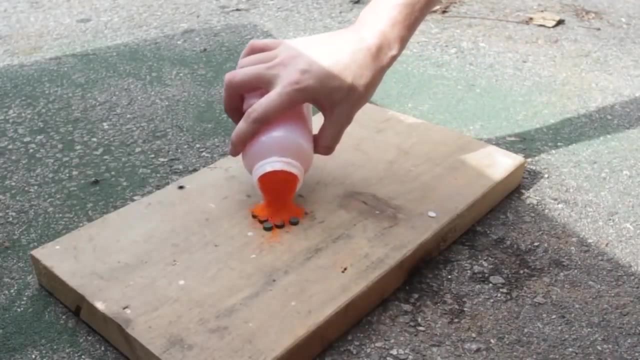 So what do you think? Thumbs up. Let's try this again, And I'm gonna make it a little bit brighter So we can see better. Let's do this again, but double the recipe And pour it right on top of it. Let's light up the top and let's see what happens.